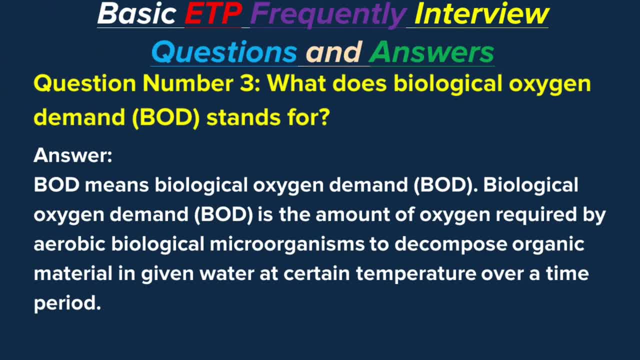 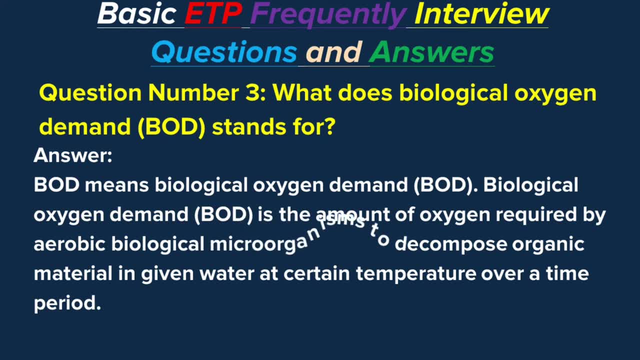 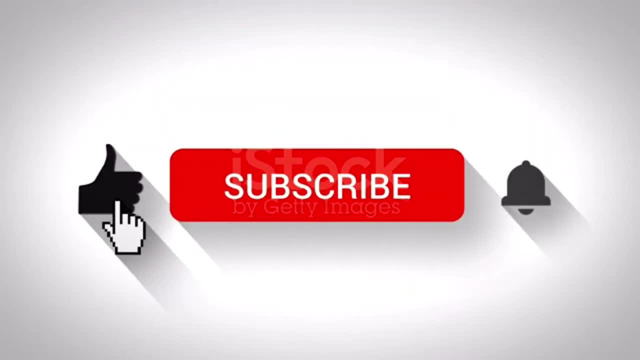 BOD means Biological Oxygen Demand is the amount of oxygen required by aerobic biological microorganisms to decompose organic material and given water at certain temperature over a time period. If you new in these channel, please subscribe channel and click the bell icon for update Notification video. 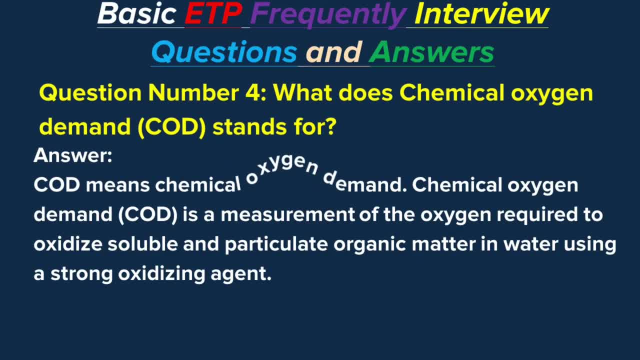 Question number 4,. What does Chemical Oxygen Demand COD stands for Answer? COD means Chemical Oxygen Demand, BOD. Question number 4, what does Chemical Oxygen Demand? COD stands for Answer? COD means Chemical Oxygen Demand, COD. 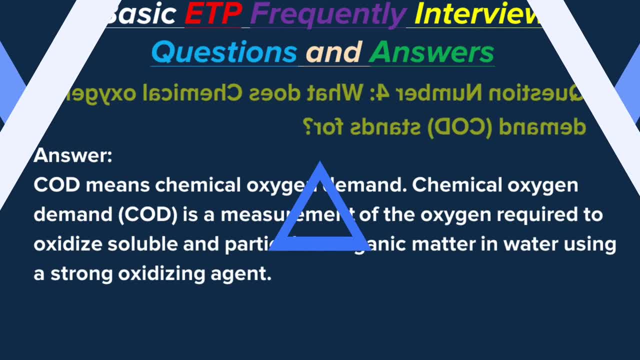 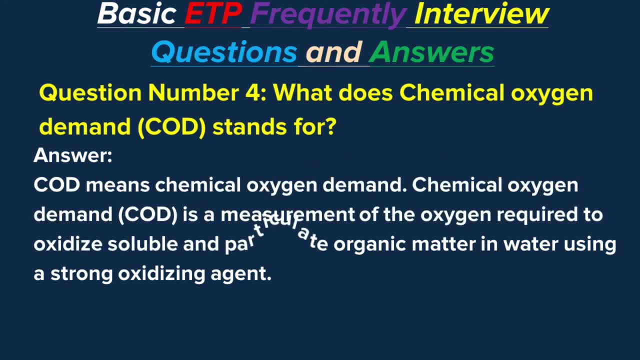 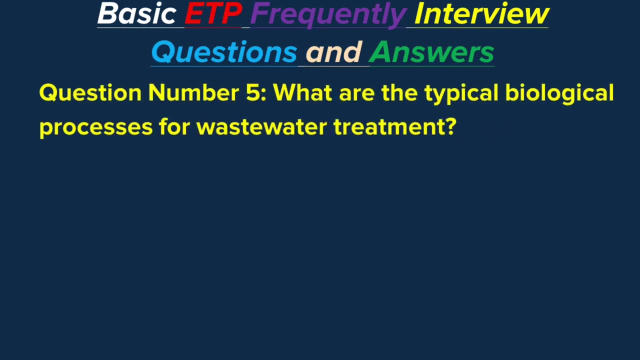 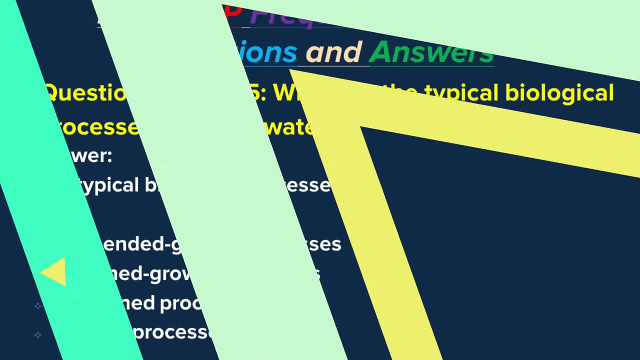 demand. chemical oxygen demand. cod is a measurement of the oxygen required to oxidize soluble and particulate organic matter in water using a strong oxidizing agent. question number five: what are the typical biological processes for wastewater treatment? answer: the typical biological processes for wastewater treatment are suspended growth. 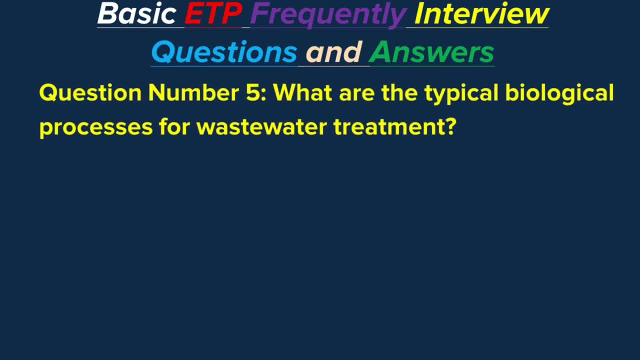 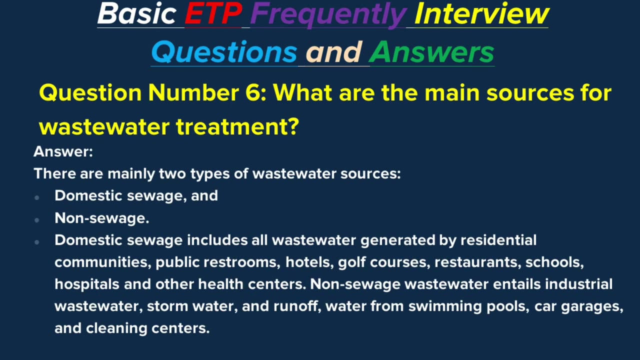 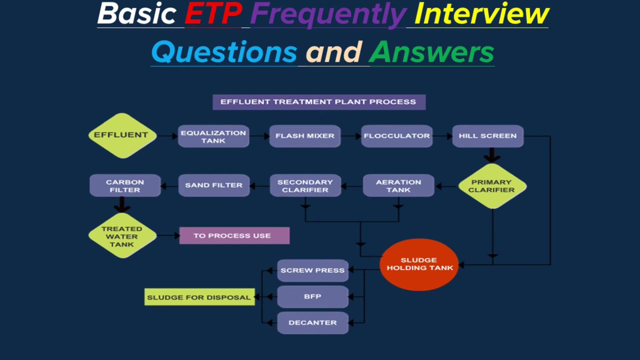 processes attached: growth processes, combine processes, lagoon processes. question number six: what are the main sources for waste water treatment? answer: there are mainly two types of wastewater sources: domestic sewage and non-sewage. domestic sewage includes all waste water generated by residential communities, public restrooms, hotels, golf courses, restaurants. 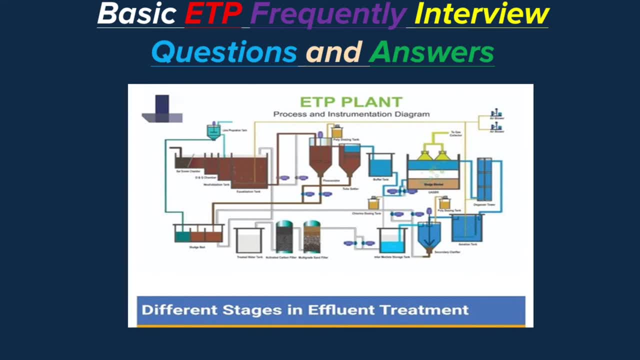 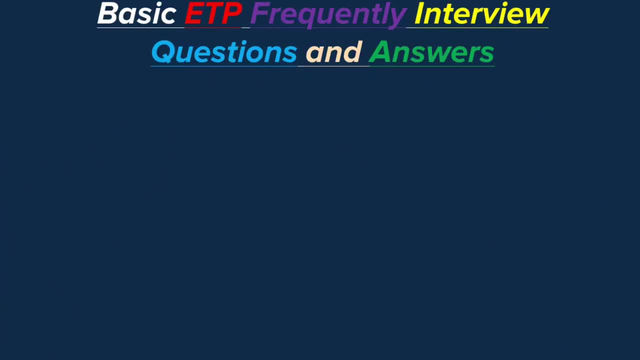 systems in machine labor, recruitment or pasture production. a mixture of wildfires and soil abstracts. there are also external waste water processingיוự to add to waste water schools, hospitals and other health centers. Non-sewage wastewater entails industrial wastewater, stormwater and runoff water from swimming pools, car garages and cleaning centers. 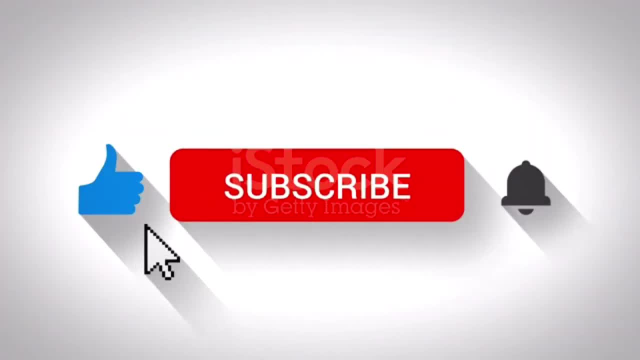 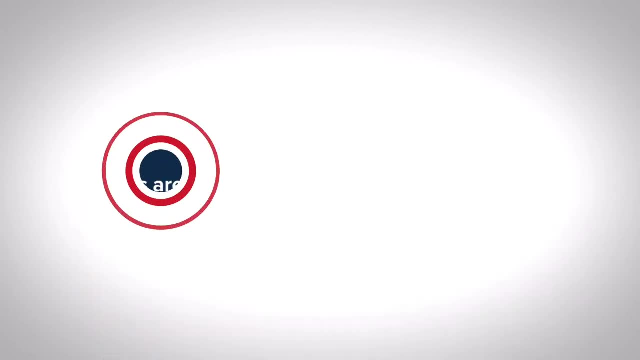 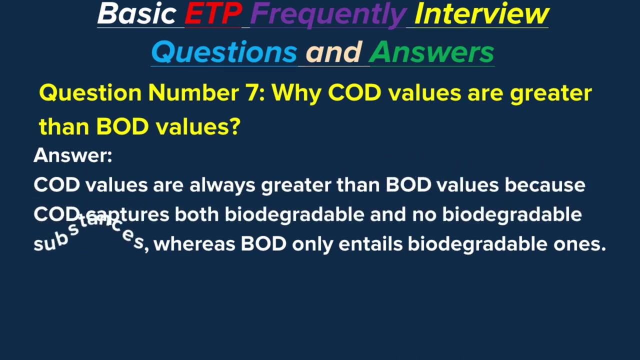 If you new in these channel, please subscribe channel and click the bell icon for update notification. video Question number 7.. Why COD values are greater than BOD values? Answer: COD values are always greater than BOD values because COD captures both biodegradable and no biodegradable substances. 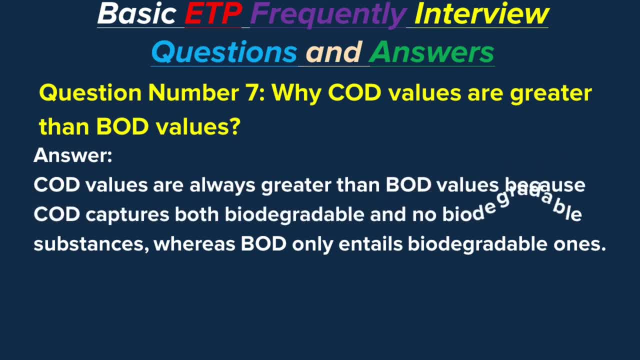 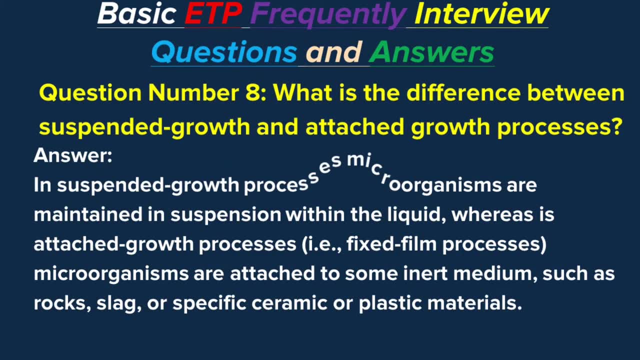 whereas BOD only entails biodegradable ones. Question number 8.. What is the difference between suspended growth and attached growth processes? Answer: In suspended growth processes, microorganisms are maintained in suspension within the liquid, whereas as attached growth processes, ie fixed film processes-